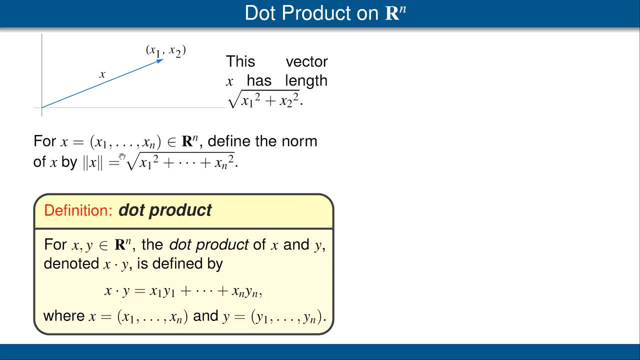 to be the sum of the coordinate y's products, as shown here. We see immediately that xx equals the sum of the squares of the coordinates. Thus xx is equal to the square of the norm of x. Now let's look at some easy properties of the dot product. 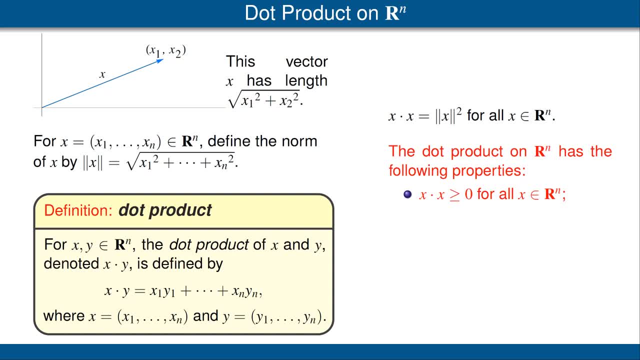 If x is a vector in Rn, then xx is bigger than or equal to zero. We also see that xx is equal to zero if, and only if, x is a zero vector. Here's a crucial property: If x is a zero vector, 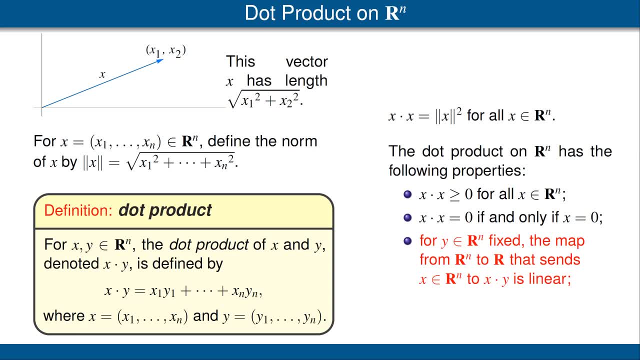 If we fix a vector y in Rn, then the map from Rn to R that sends x to xy is linear. In fact, this is the reason we introduced the dot product. We're bringing some linearity- which is always useful- back into the picture. 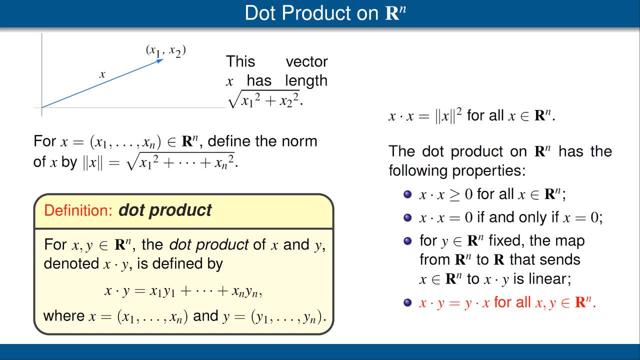 And the final easy property: If x and y are vectors in Rn, then xy is equal to yx. In other words, the dot product is commutative. Note that the dot product of two vectors in Rn is a number. it's a real number. 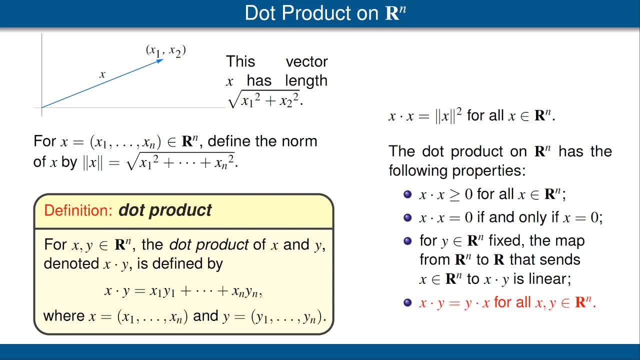 The four properties of the dot product on Rn shown in the four bullet points here are almost what we want to abstract to get to the notion of inner product. In fact this works perfectly on real vector spaces, but for complex vector spaces there's 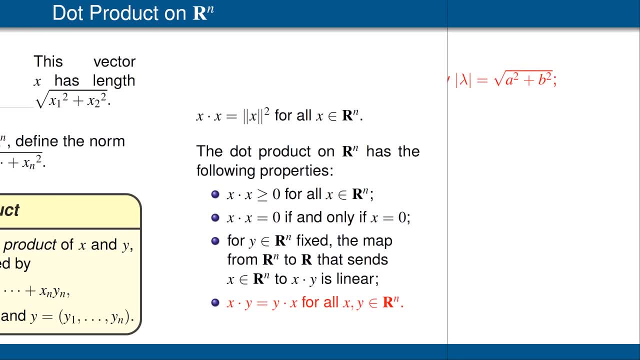 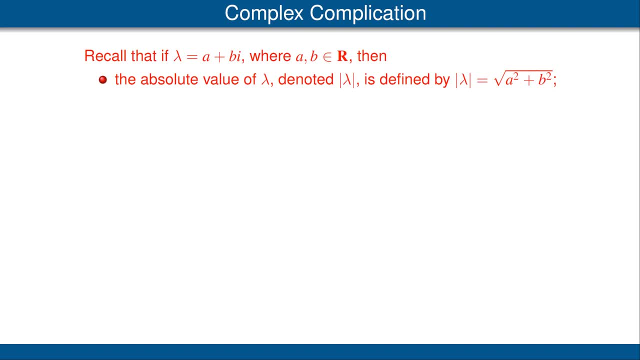 a little bit of a wrinkle that we need to consider. first, Recall that if lambda is a complex number, then the absolute value of lambda is defined to be the square root of the sum of the squares of the real part of lambda and the imaginary part of lambda. 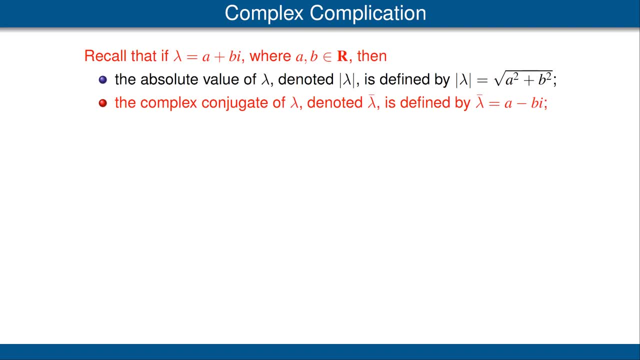 The complex conjugate of lambda is defined by multiplying the imaginary part by negative 1.. And we have the extremely useful identity that the absolute value of lambda squared is equal to lambda times the complex conjugate of lambda. For z, a vector in Cn, we define the norm of z to be the square root of the sum of the. 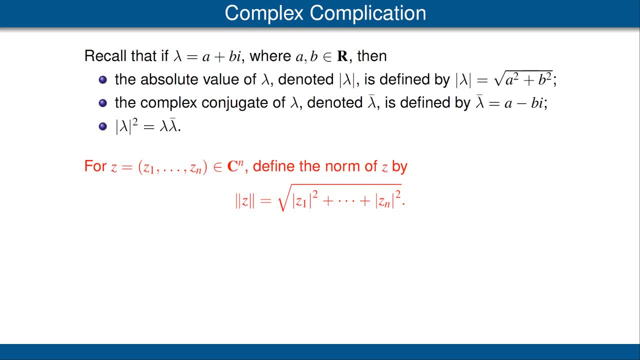 squares of the absolute values of the coordinates. Note that we're squaring the absolute values of the coordinates, not just the coordinates themselves. This is because we want the norm to end up being a non-negative number. When we were working on Rn, we did not need to bother with absolute values when computing. 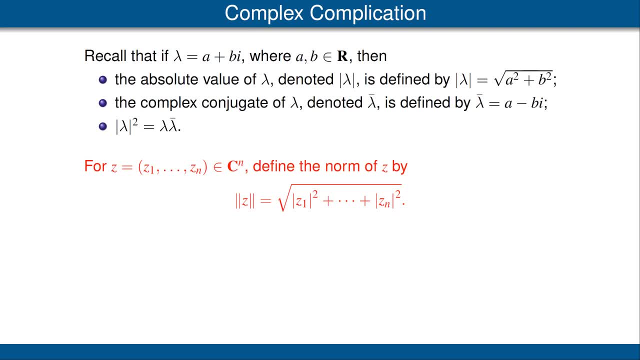 the norm, because the square of any real number is the sum of the squares of the absolute values of the coordinates. If we want to recover the relationship between the norm and the inner product, then we can no longer use our previous definition. The definition of norm in Cn suggests that our inner product of a vector w and z should: 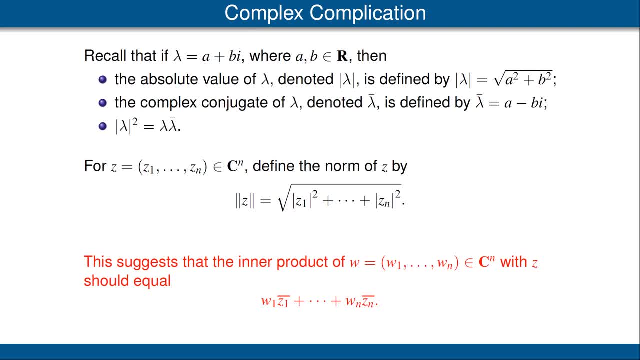 be obtained by multiplying together the coordinates, but taking the complex conjugate of the second vector and then adding up as shown here. This provides our final motivation for the definition of an inner product. Please keep this in mind as we go to that definition now. 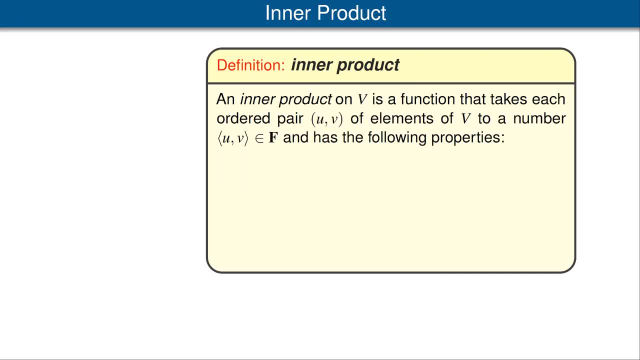 We are now ready to give our definition of inner product. As usual, we will give a definition that works simultaneously, regardless of whether the scalar field F is equal to the real numbers or whether it is equal to the complex numbers. Here we go: An inner product on our vector space. 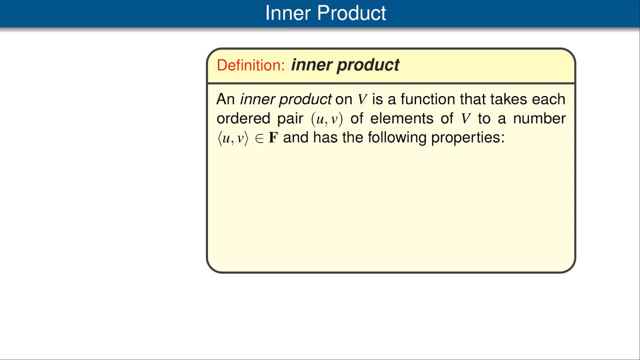 v is a function that takes each ordered pair of elements, u comma v in v to a number which we denote by u comma v, with angle brackets around them. that has the following properties: The first property is that the inner product of a vector with itself should be a non-negative. 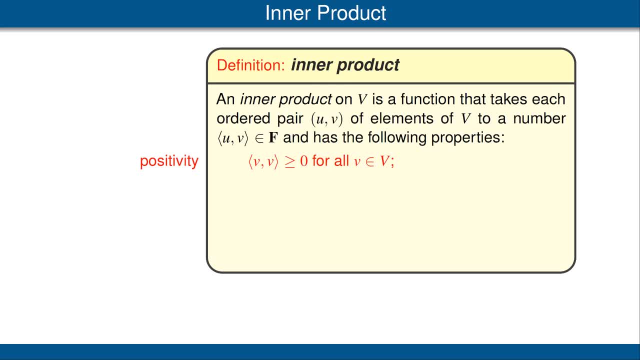 number. By the way, when we use the greater than or equal to sign with a number that could conceivably be complex, we mean that the number is real and non-negative. Our second property is that the inner product of a vector with itself is equal to zero if. 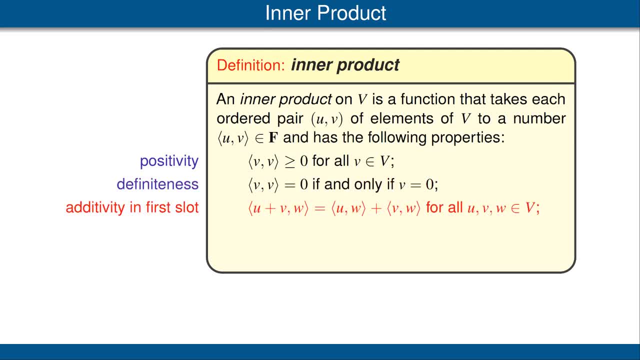 and only if the vector is zero. Our third property is called additivity in the first slot. This means: fix a vector w, it will go in the second slot, and then we have the additivity property shown by the equation here. The next property is called homogeneity in the first slot. Again, fix a vector in the. 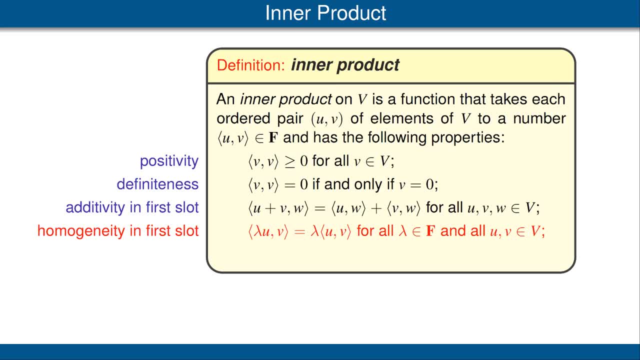 second slot. and then we have the equation shown here, which indicates that if we have a scalar times a vector in the first slot, then we can bring the scalar outside. Our last property in the definition of an inner product is called conjugate symmetry. 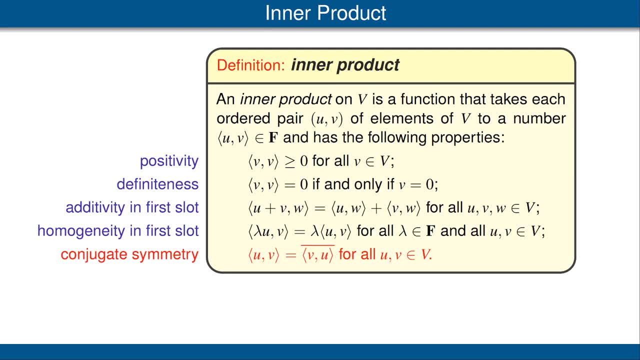 It says that if we interchange the order of the two vectors, we get the complex conjugate of what we started with. Recall that the complex conjugate of a real number is just the real number itself. Thus, in the case where our scalar field f is the field of real numbers, this property 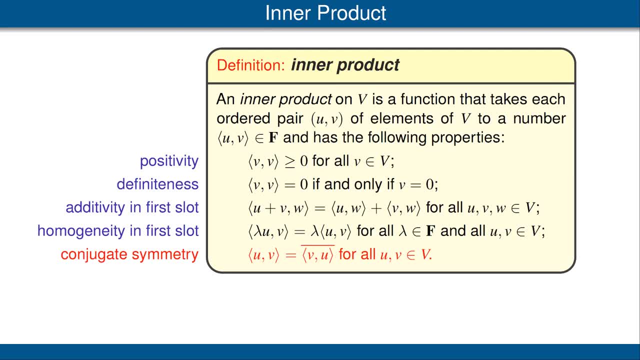 could be rewritten to say: the inner product of u with v is equal to the inner product of v with u. In other words, when dealing with real numbers, the complex conjugate does nothing. However, it will matter when we are dealing with complex numbers. We leave it here. so 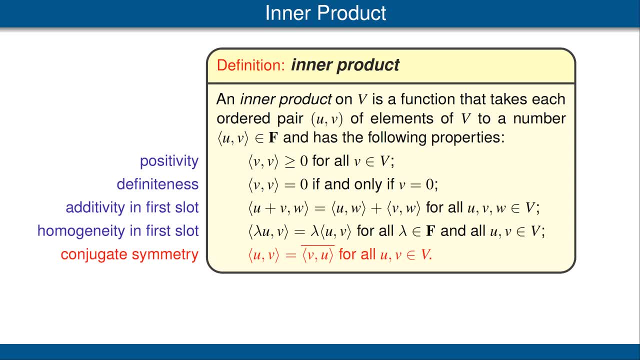 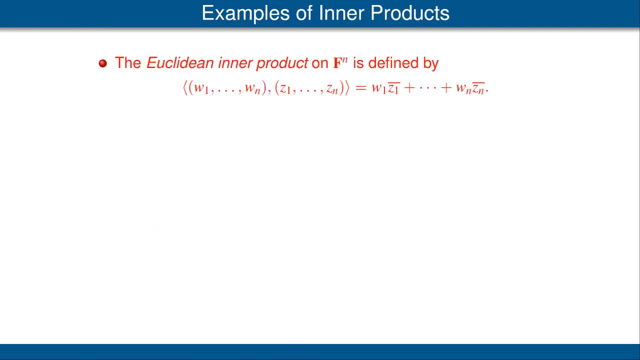 that we can have a single definition. Now let's look at some examples of inner products. For our first example, a vector space will be fn and we have what is called the Euclidean inner product. As you can see, if f happens to be the scalar field of real numbers, this inner product. 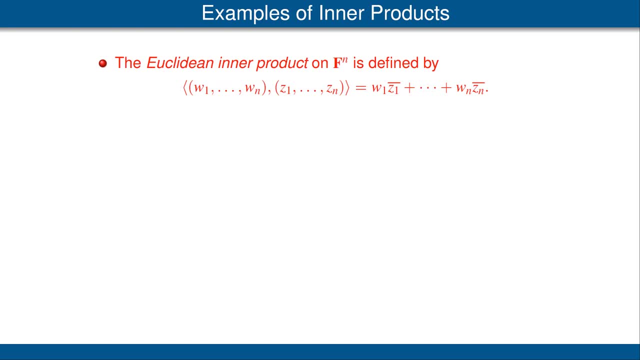 agrees with the dot product that we had defined earlier. Here is another example of a scalar field of real numbers. Here is another example of a scalar field of real numbers. For our next example, a generalization of the first one, suppose we take positive numbers. 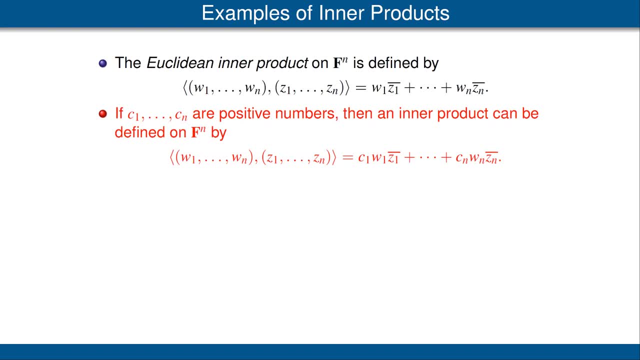 c1 up to cn, then we can define an inner product on fn, as shown by the equation here. If all the c's are equal to 1, then we have the example from the first bullet point. For our next example, consider the real vector space consisting of the continuous real-valued. 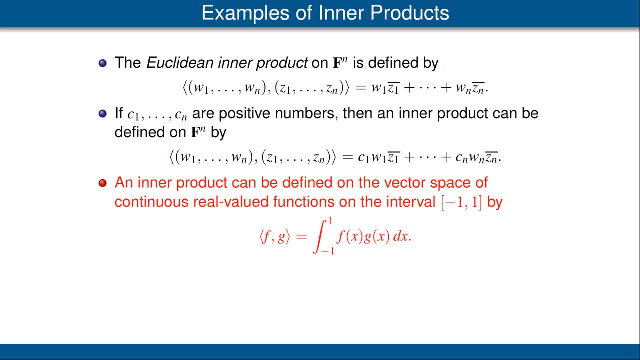 functions on the interval from minus 1 to 1, and define the inner product of two functions, f and g, to be their integral. You should pause the video for a moment to verify that this definition of inner product satisfies all four required properties for an inner product. 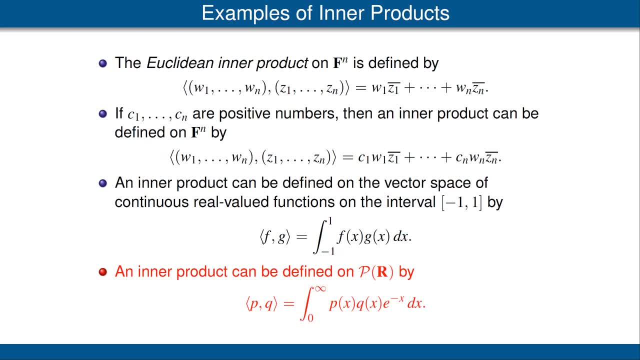 For our final definition. we'll again look at a real vector space, this time the vector space of polynomials with real coefficients. We define the inner product of two such polynomials to be the integral, from 0 to infinity, of the product of the polynomials times, the function e to the negative root of 0.. 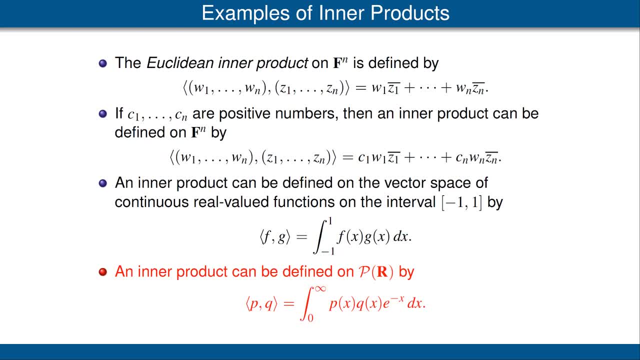 The integral is the integral from 0 to infinity of the product of the polynomials times the function e to the negative root of 0. x. This integral converges and makes sense because e to the negative x goes to zero much faster, as x goes to infinity, than any two polynomials can. 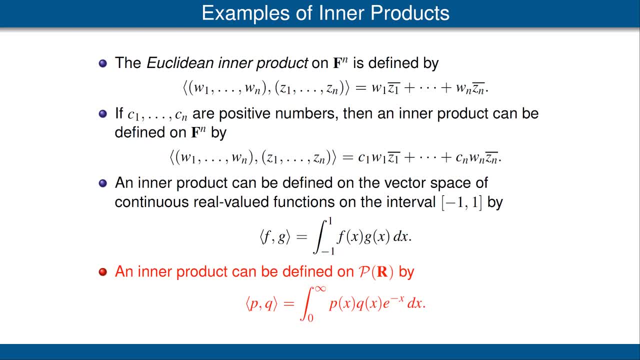 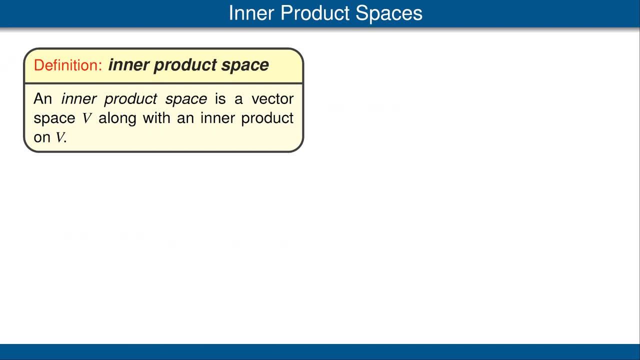 grow. The key point for all four of these examples is that an inner product is a function depending upon a vector space, and it gives us for each two vectors in that vector space, a scalar. When we call something an inner product space, we mean that it is a vector space along with an inner product on it. Until further notice, 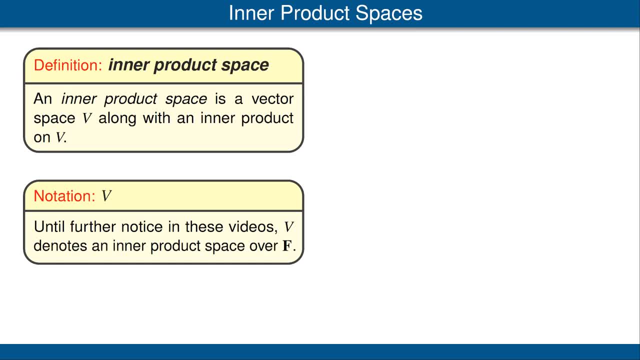 in these videos we will let v denote an inner product space over f. By making this a standard assumption, we will not have to repeat in the hypothesis of each result that v is an inner product space. Now let's look at some properties of inner product spaces. Here's our first property. Suppose we fix a vector u in v. 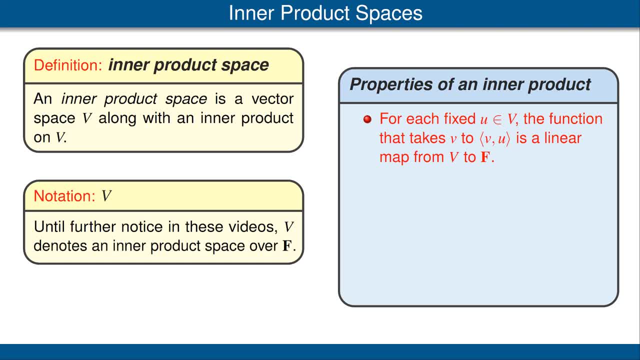 Then the function that takes a vector in v to that vector inner product with u is a linear map from v to f. This linearity follows from additivity in the first slot and homogeneity in the first slot. Our second property says that the inner product of zero with any vector in 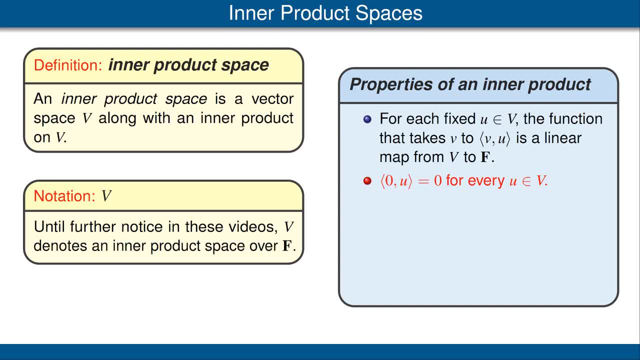 v is zero. That follows immediately from linearity. Our third property says that the inner product of any vector with zero- now with zero in the second slot- gives us zero. We obtain that result from the second bullet point by using the property that if we interchange the order of two vectors, 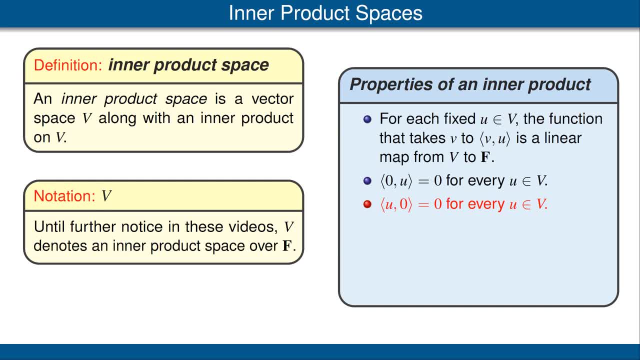 when taking an inner product. then we get the complex conjugate And of course the complex conjugate of zero is equal to zero. Our next property is called additivity in the second slot. This can be proved by using additivity in the first slot along with the property that interchanging the order gives. 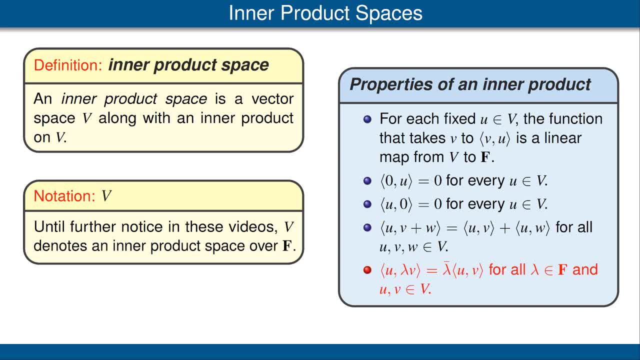 us the complex conjugate. And our last easy property states that if we have a scalar multiple of the vector in the second slot than the scalar comes out multiplied by a complex conjugate. Again, this property follows from the definition, using its properties, that interchanging the order gives you the complex conjugate.